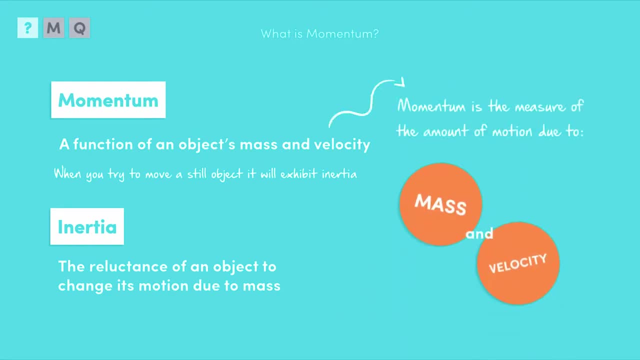 Momentum is a measure of the amount of motion due to mass and velocity. If either of those two things increase, then the momentum increases as you have, overall, more motion if you're either larger or if you're going faster. So the actual calculation, rather than these just vague general ramblings of mine: momentum: 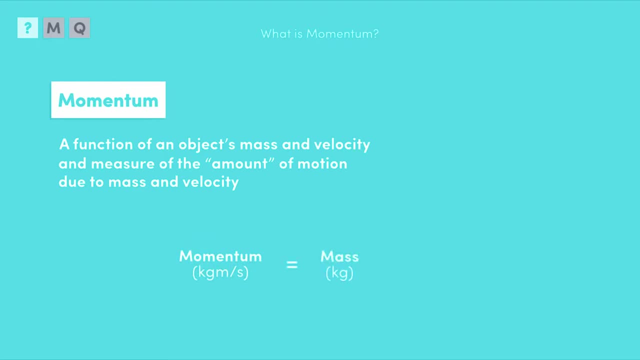 in kilogram metres per second equals mass in kilograms times velocity in metres per second, or p equals mv. Notice how it is a lowercase p, not capital P, like pressure. It's pretty obvious when you look at it that if you either increase your mass or your velocity, then you increase. 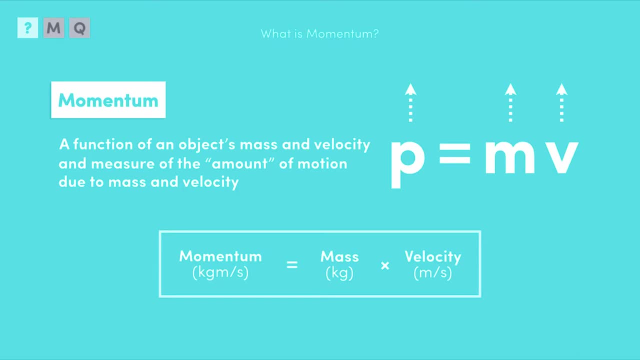 your momentum. One thing to note is that, as well as donating its magnitude, velocity also comes with the baggage of being a vector, so there's a direction coming along as well That, unfortunately, because it's more complicated, also makes momentum a vector. So, alas, we have to keep. 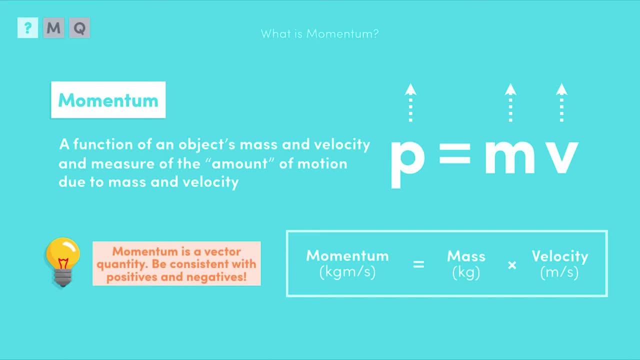 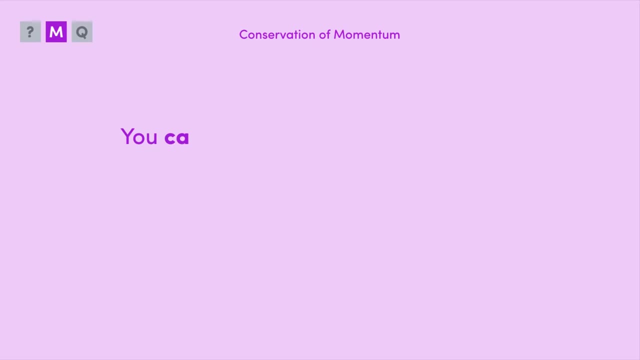 our directions in check for all these problems. The fundamental principle I talked about, Like I said with you, can't create or destroy energy in any interaction. momentum is conserved. Well, momentum is conserved with a big old asterisk. Energy is always conserved, but momentum comes with a wee caveat: Momentum. 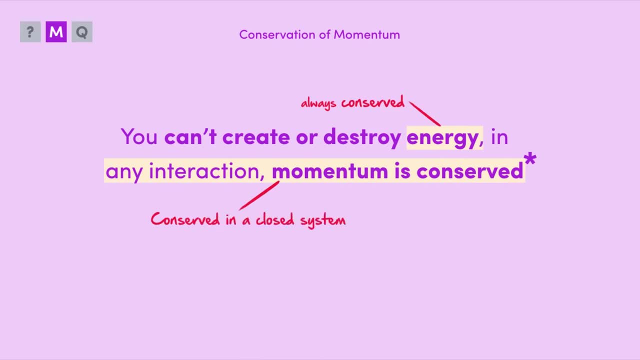 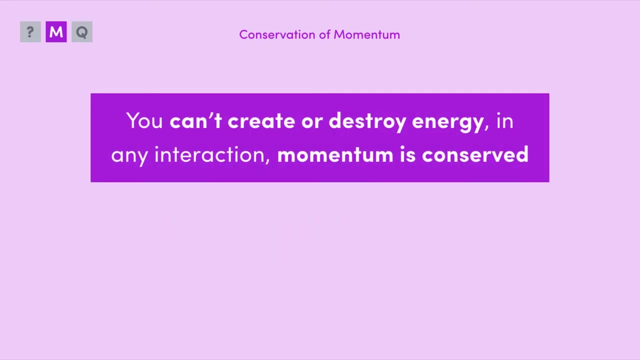 is conserved in any interaction in a closed system, ie no external forces acting which cause a change in momentum. We'll be talking about changing the overall momentum in the system using forces in the next video. So if you don't have an external force acting, then you can always say that the total momentum 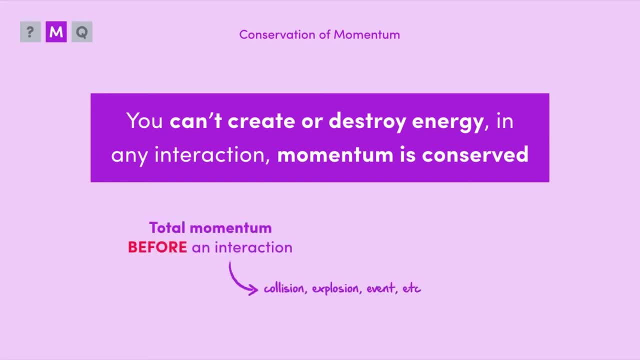 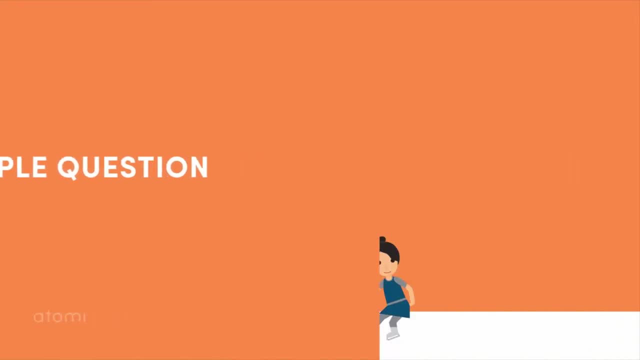 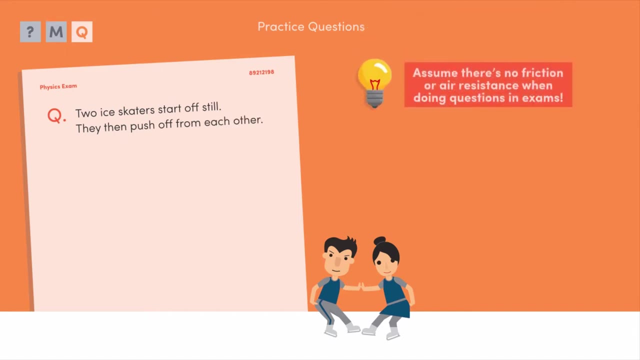 before an interaction, say a collision or an explosion or something like that, will be the same after the interaction. So let's say you have two ice skaters. They start off still and then push off from each other. We're assuming no friction or air resistance etc. etc. like we do in most of the 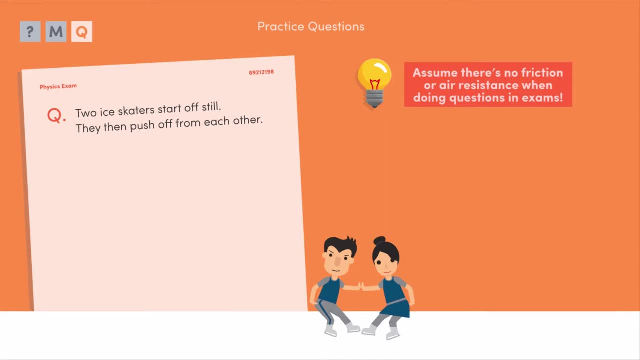 time in these mathematical situations. But anyway, here is the question. The male skater has a mass of 90kg and the female skater has a mass of 60kg. When they push away from each other, the male skater moves left with a velocity of 2.5 meters per second. What is the velocity? 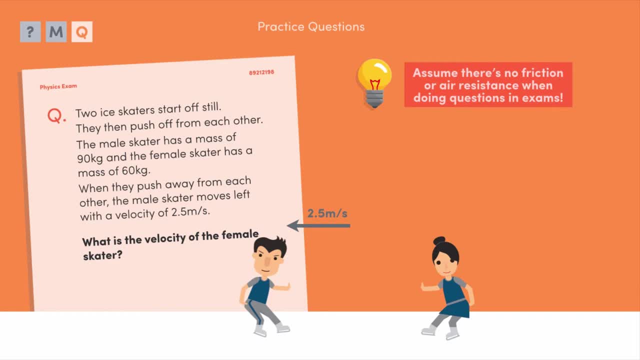 of the female skater Right. so again, lots and lots of words and you need to pull out the numbers you need. The way I always set this out is in two columns like this: A before column and an after column. We know straight from the question that the momentum before equals. 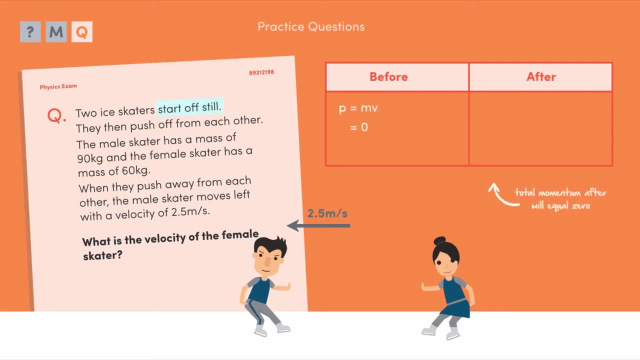 zero because nobody and nothing is moving. So afterwards the total momentum has to equal zero because momentum is conserved. Obviously each skater has a non-zero momentum because they're now moving, but the total momentum in the situation remembering that momentum. 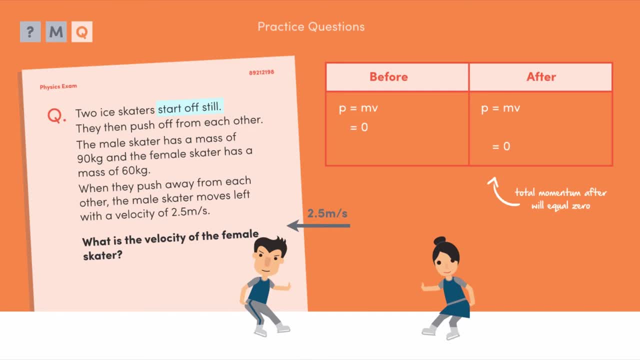 is a vector has to equal zero. So the momentum of the male skater here has to cancel out the momentum of the female skater. So the columns look like this Because we're just adding the two momentums together. we can say that 90 times 2.5 plus 60 times unknown. 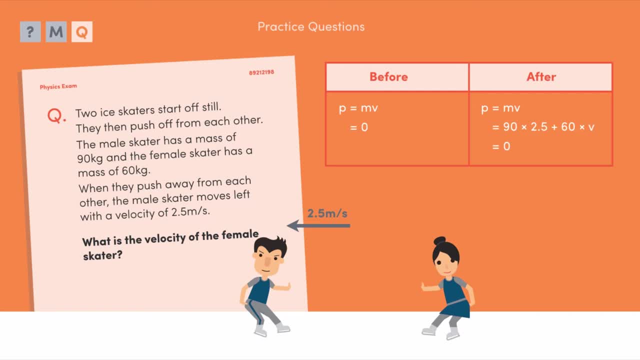 velocity equals zero. Rearranging the after equation gives you velocity equals minus 3.75 metres per second. It's negative, which is great. We expect that, since, in order to cancel out the momentum of the male skater, we're going to have to cancel out the momentum of. the female skater. So the columns look like this Because we're just adding the two momentums together. we can say that 90 times 2.5 plus 60 times unknown velocity equals zero. Rearranging the after equation gives you velocity equals minus 3.75 metres per second. It's negative. 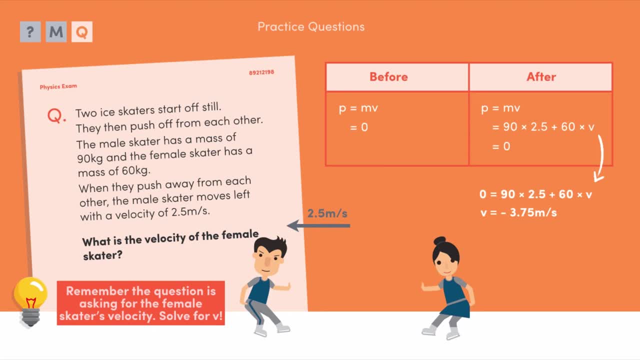 which is great. We expect that, since, in order to cancel out the momentum of the male skater, the female skater has to be going in the other direction, You could leave it as negative in your answer. or, since the question tells you the male skater moves left, you could. 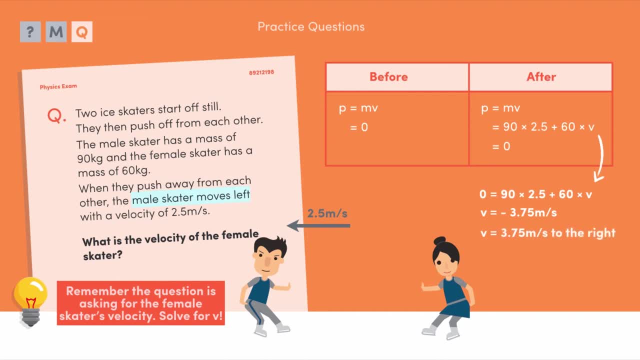 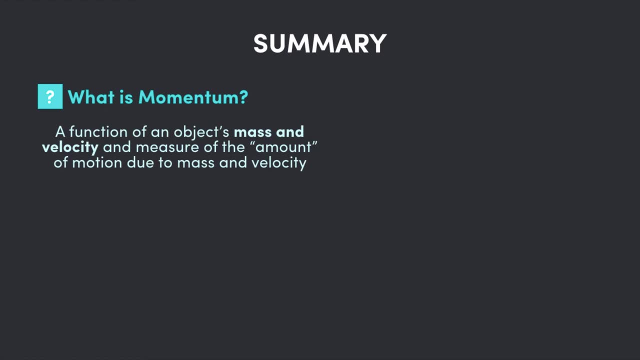 just say: v equals 3.75 metres per second to the right. Okay, so that's. that Definition of momentum is a bit of a weird one, but you are very much within your rights to just quote the equation in the exam, as long as you define. 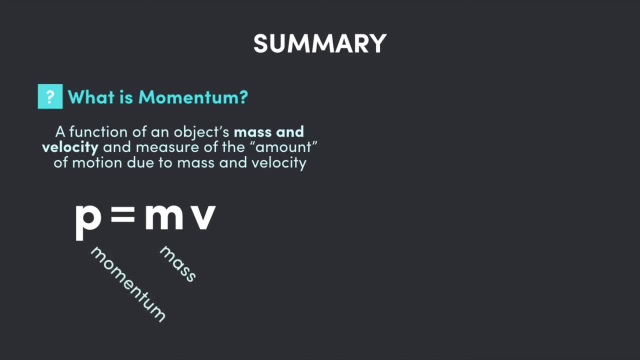 all the variables say: p equals momentum, m equals mass and v equals velocity. The idea that momentum is conserved isn't a particularly difficult one, but it's the directions and the positives and the negatives that get everybody tied up in knots. so again,